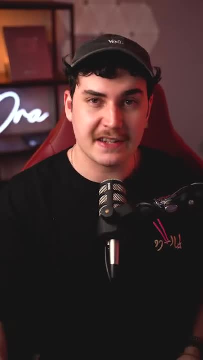 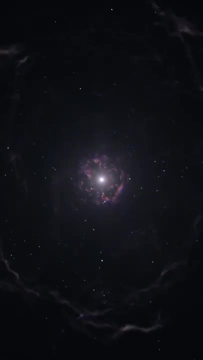 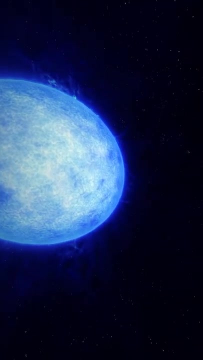 Neutron stars are sometimes called the most extreme objects in the universe other than black holes, and it's for good reason. They are the collapsed cores of supergiant stars, 10 to 25 times the mass of our sun. They are roughly 20 kilometers in diameter, but have 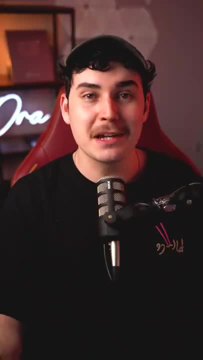 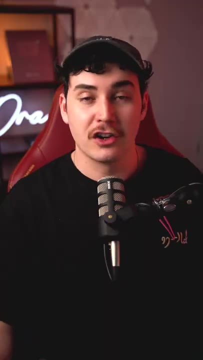 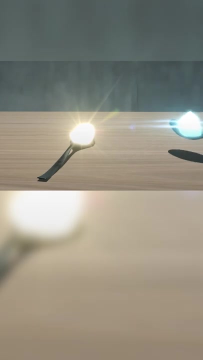 nearly 1.5 times the mass of the sun. I mean, think about that, all of the mass from the sun and more, squished down into the size of just a few suburbs. For context, if you took a teaspoon of matter from the sun, it would weigh around 2 kilograms. but if you took a teaspoon of 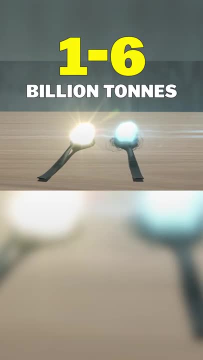 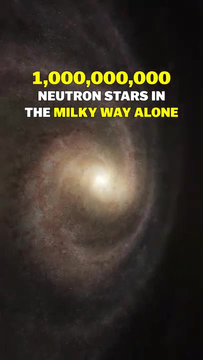 a neutron star, it would weigh somewhere between 1 and 6 billion tons. And what's crazier, we think there is around 1 billion neutron stars in our Milky Way galaxy alone. Space is crazy. 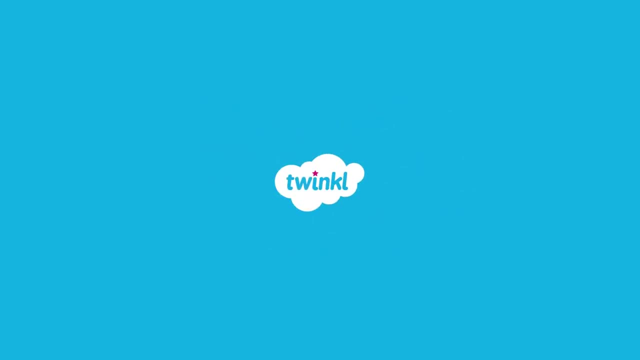 Do you recognise all of these coins? Do you hear something? The piggy bank is rattling. It's 1p. This coin isn't worth a lot. In fact, one pence is the lowest value coin. Let's see what else our piggy bank has inside it. That's 2p. Did you know that two 1ps are? 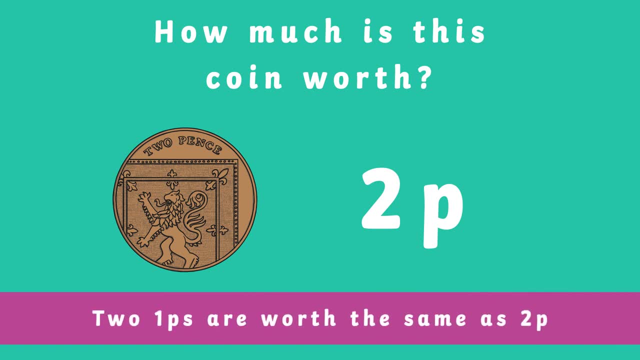 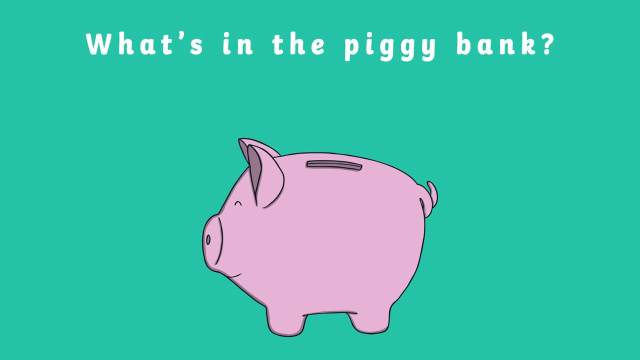 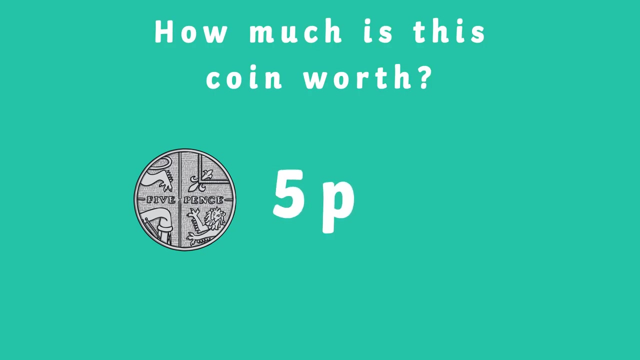 worth the same as 2p. Did you know that two 1ps are worth the same as 2p? Did you know that two 1ps are worth the same as 2p? What coin is up next? It's 5p. 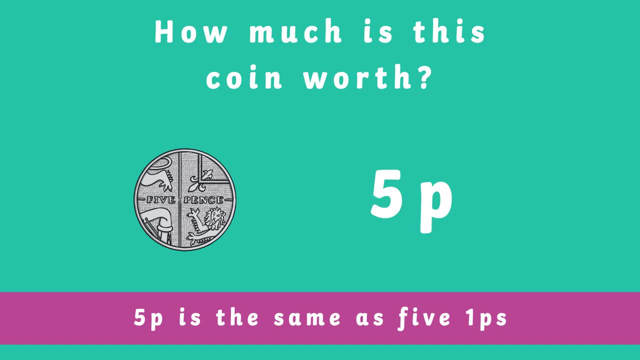 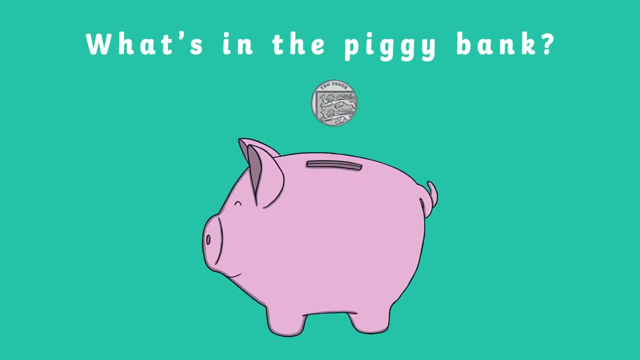